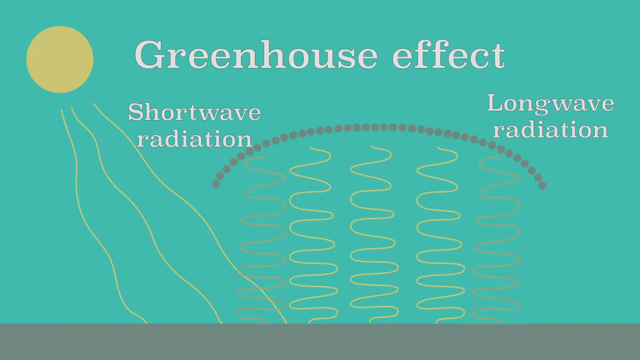 Just like a greenhouse. the heat can easily enter the atmosphere, but it's hard for the heat to leave the atmosphere. You could compare this to a car with the sun shining in. The heat can easily go in, but the heat can't leave the car. 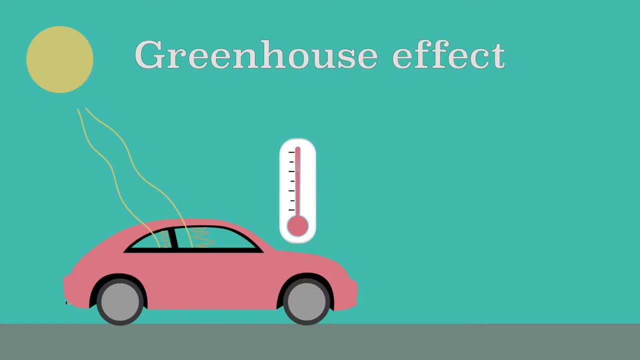 which causes the car to heat up very quickly. Without the greenhouse effect, it would be around 30 degrees colder on earth, So it's a good thing that this effect exists. However, more greenhouse gases are released into the atmosphere through the emission of exhaust gases. 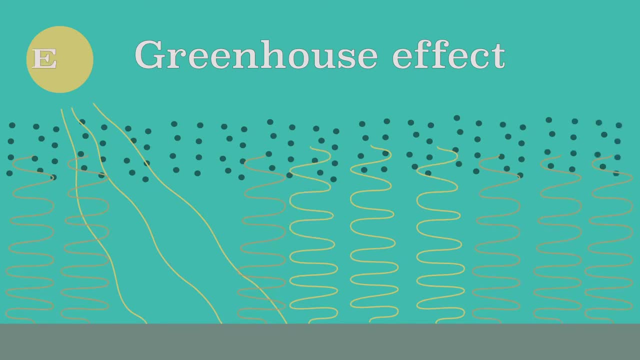 This makes the greenhouse effect stronger. This is therefore referred to as the enhanced greenhouse effect. Among other gases, carbon dioxide, which is often abbreviated to CO2,, is responsible for this. The amount of CO2 in the atmosphere differs per season. The amount of CO2 in the atmosphere differs per season. There is more land in the northern hemisphere and therefore more trees. In the summer months, they absorb a lot of CO2, reducing the CO2 content in the atmosphere. At the end of the summer, the CO2 content in the atmosphere increases again as leaves are broken down. 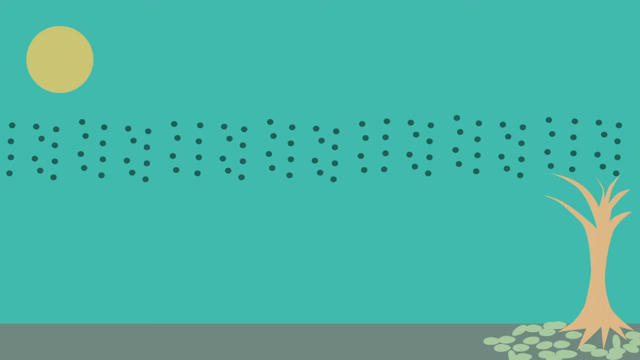 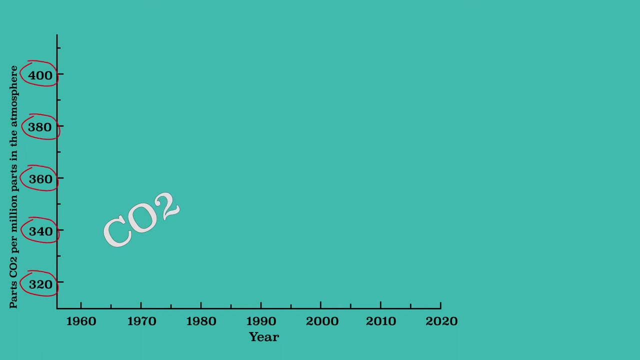 Nature therefore also has a major influence on the amount of CO2 in the atmosphere. The amount of CO2 is measured by the number of CO2 particles in the atmosphere per million gas particles in the atmosphere. There are also many other gases in the atmosphere. 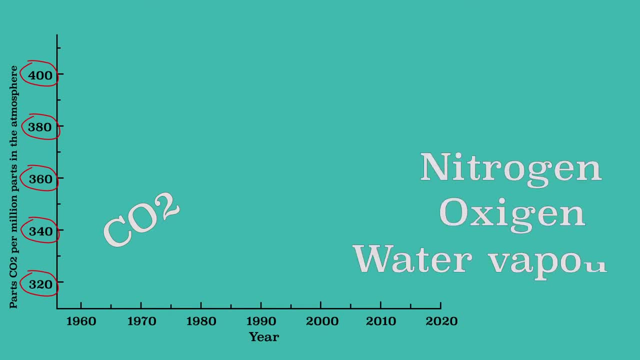 such as nitrogen oxygen and water vapor. About 250 years ago, there were 277 parts of CO2 per million particles. Now there are 404, and this number is growing every year, Although 400 CO2 particles per million does not seem very much. 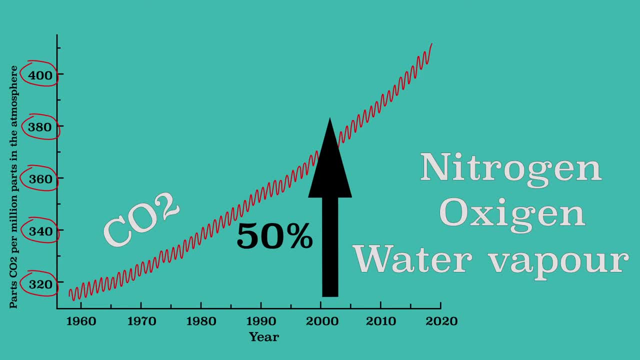 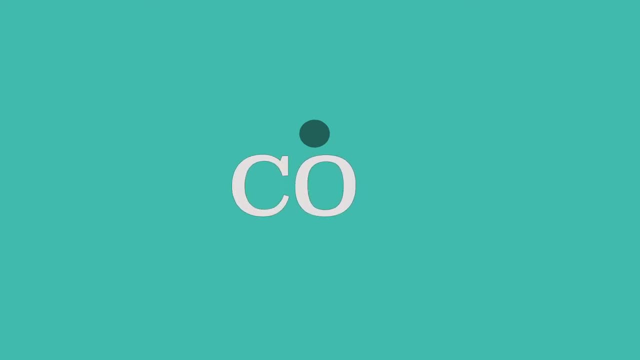 the increase is almost 50% and this can have a major effect on processes in the atmosphere. Let's see where that extra CO2 comes from. The C in CO2 stands for carbon. Carbon occurs in the atmosphere in two forms, which we call C12 and C13. 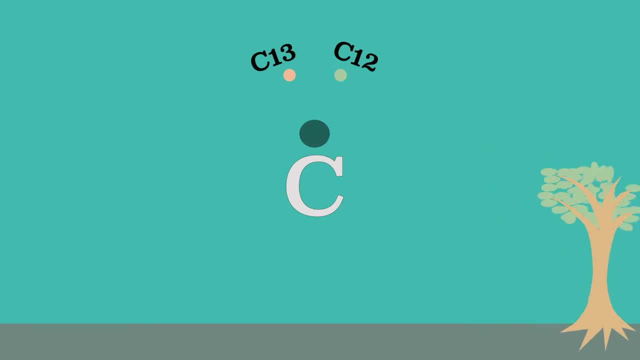 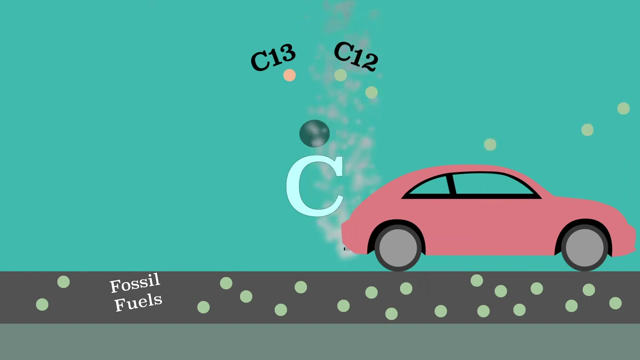 C12 is lighter and plants therefore prefer to absorb C12.. Plants, and ultimately fossil fuels, therefore contain a relatively large amount of C12.. We see that the ratio between C12 and C13 in the atmosphere is changing. This is because proportionally more and more C12 enters the atmosphere.